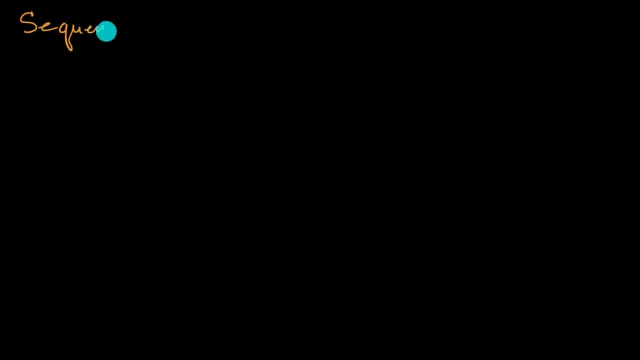 The focus of this video is going to be on sequences which you have hopefully already seen. If you don't know what a sequence is, I encourage you to review those videos on Khan Academy. But we're going to focus on how we can generate. 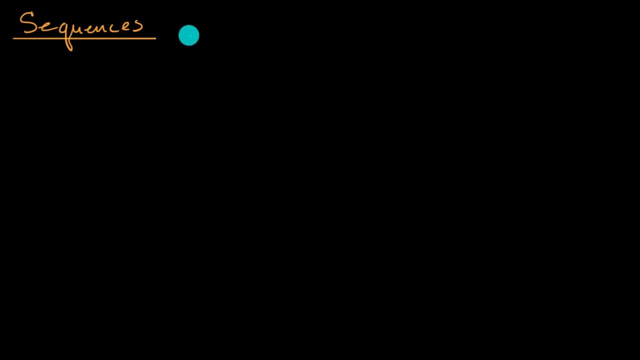 the same sequence with different functions that have different domains. So let's just start with an example sequence. Let's say we have a sequence, It's a six. you could call that the first term. Some people would call that the zeroth term. six: 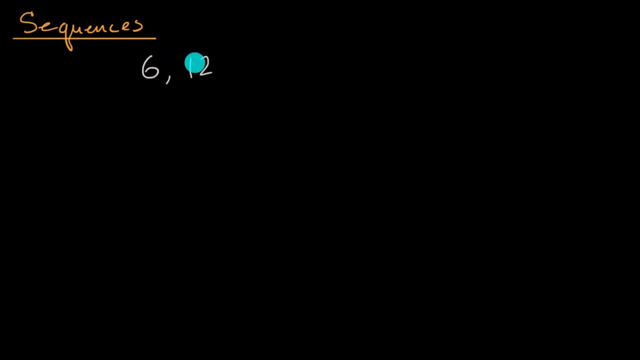 And then, if that's the first term, the second term is now a 12,, then a 24,, then a 48, and so on and so forth, And, as we'll see, there's multiple function definitions that could create the sequence. 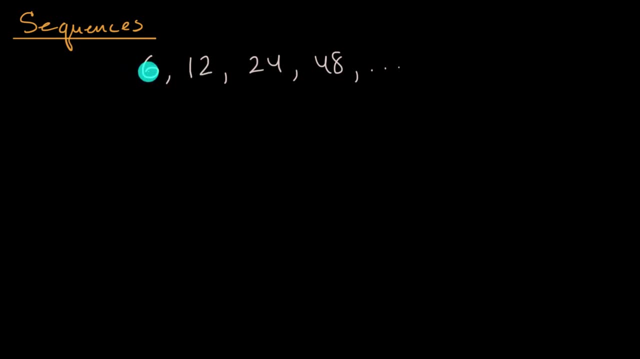 One way to think about it is: this is six times one, This is six times two, This is six times four, This is six times eight. So it looks like each term is six times eight. This is six times a power of two. 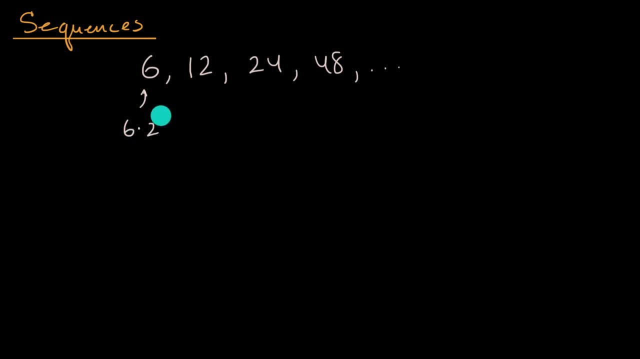 Let me make that clear: This one right over here is six times two to the zero, That's six times one. This one over here is six times two to the first. This one over here is six times two, squared Six times four. 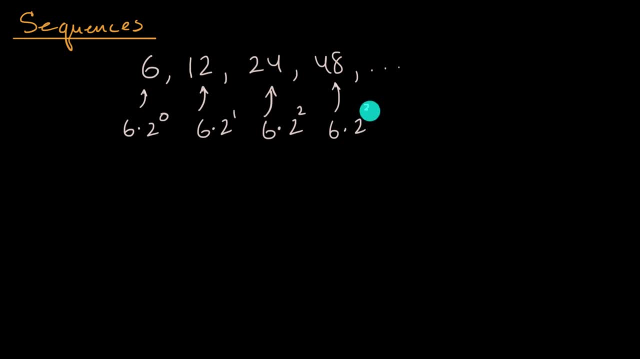 This right over here is six times two to the third, And so one way to view this is, if you view this as the zeroth term, we could define a function. call it a of n, where n is referring to our index, or which term in the sequence. 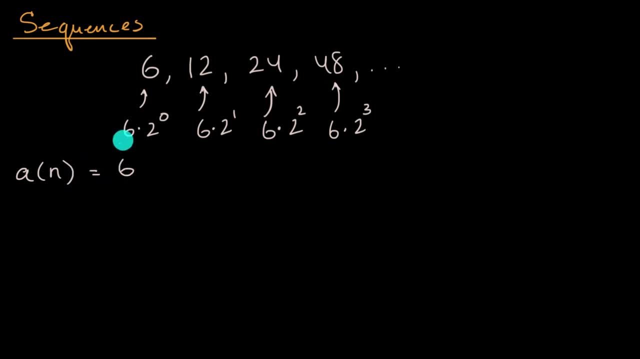 and it's equal to six times two. six times two to the n, where n starts at zero and then it keeps incrementing by one. So it's really all integers greater than or equal to zero, And it's very important to specify that domain. 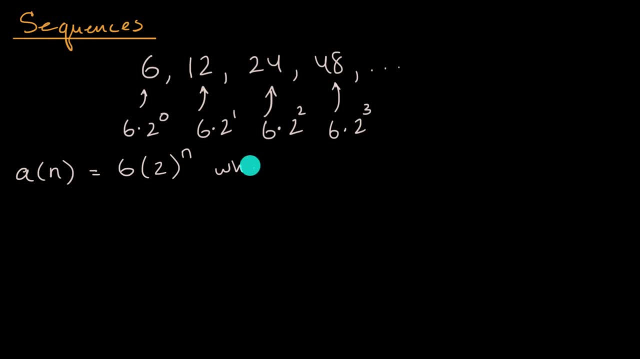 where n, where n is an integer, integer and n is greater than or equal to zero, You could see what happens if n is not an integer. If you tried to put a 1.5 here or something like that, then you're not going to get one of the terms. 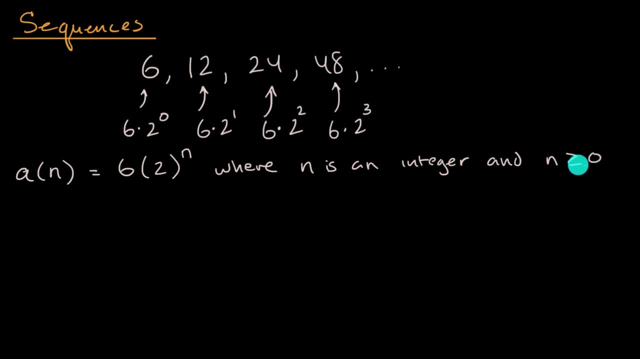 in the sequence, And if we don't start at zero, if we started at one, then this would be the first term in the sequence, which is not what we want. We wanna generate the sequence, the sequence that I originally wrote down, And obviously, if you started at n equals negative one. 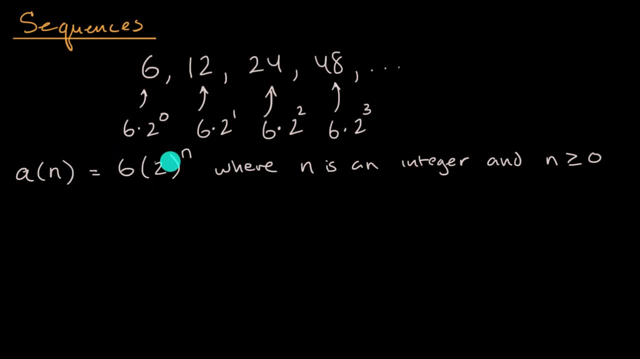 then you're gonna get a different value for your first term. So this is one way to essentially define or to create a function which generates this sequence, But, as we'll see, there are other ways to do it. For example, let me do another one. 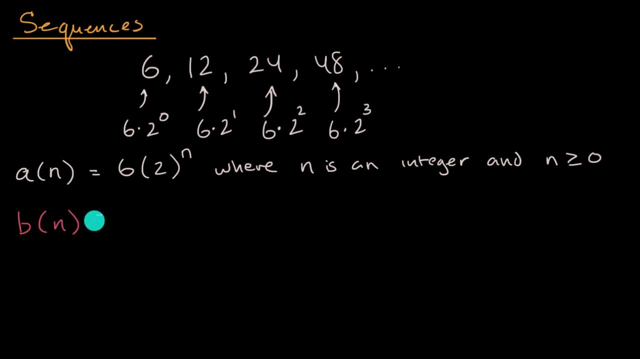 I'll do it another color. Let's say I have b of n And let's say I want to, instead of making, instead of saying okay, I'm gonna start at n equals zero, and you could kind of view this as a zero term. 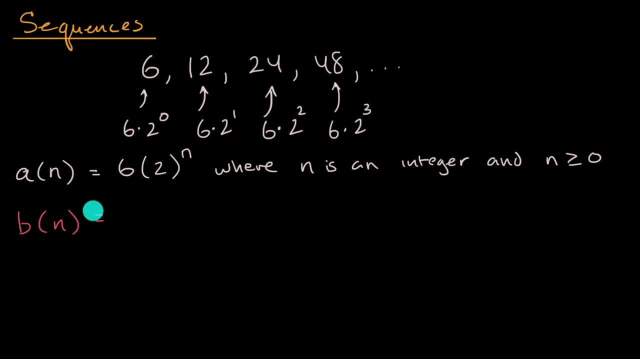 I wanna start at. n equals one. So what you could do is is, when you input a one, this essentially becomes a zero. How do I do that? Well, I just subtract one from it. So I could say six times two to the n minus one power. 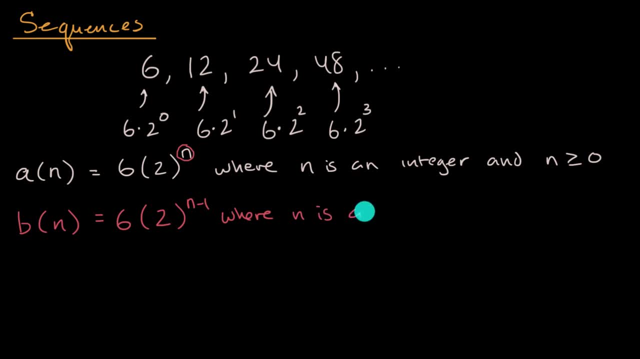 where n is an integer integer and n is greater than or equal to one. Notice now, when we put n equals one in here- and we could maybe call this the first term- we wanna generate a six. So what happens? One minus one, we get that zeroth power. 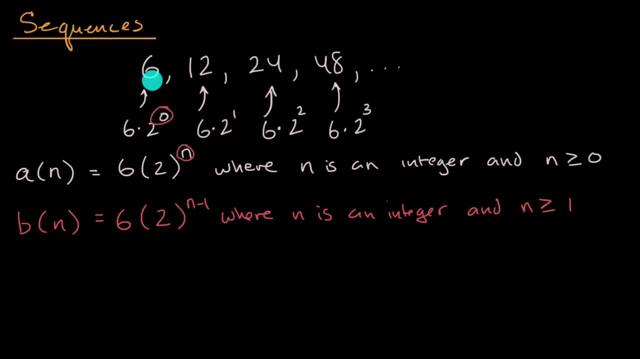 that we want right over there. And so six times two to the zero is indeed six. Then when n is equal to two, it's six times two to the two minus one, which is just two to the first power. So it's just become six times two, which is equal to 12.. 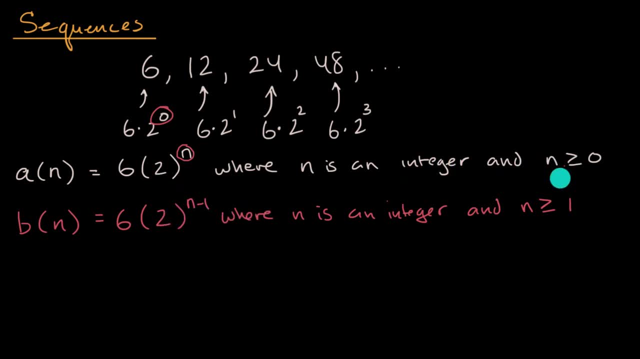 So notice these are different function definitions with different domains, But they're generating the exact same sequence. We could also do it recursively And we've seen this in other videos. We can define a function recursively. We could say: all right, look, 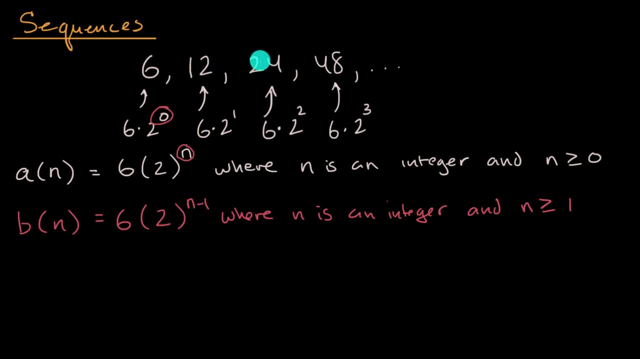 it looks like each of these, each of these terms in our sequence is twice the previous term. So we could. if we want a recursive definition for the sequence, we can define the first term Or in this case we could say the zeroth term.